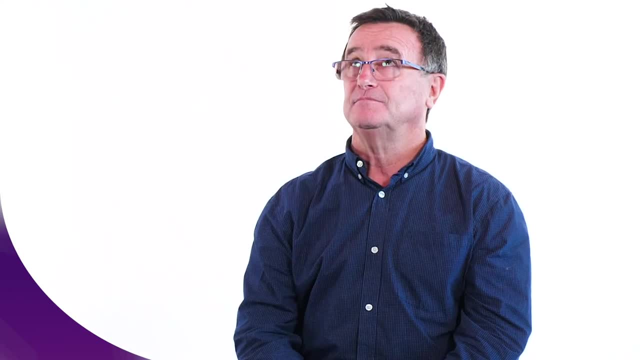 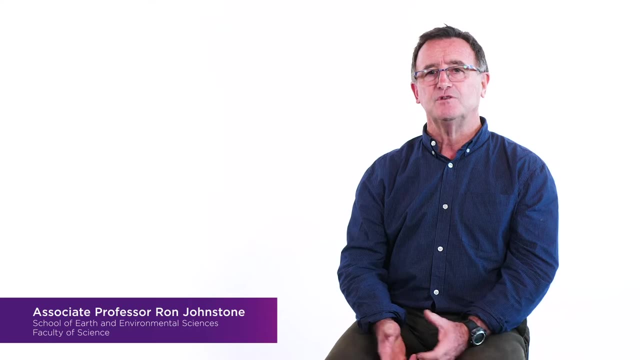 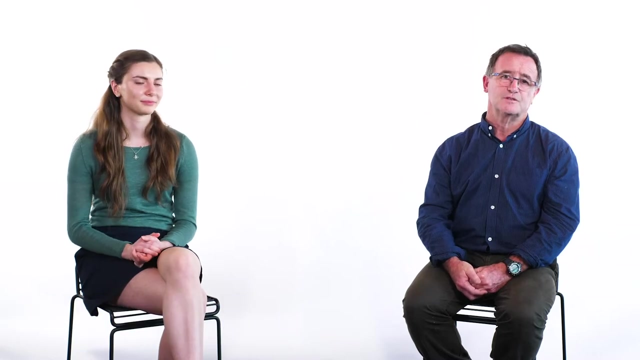 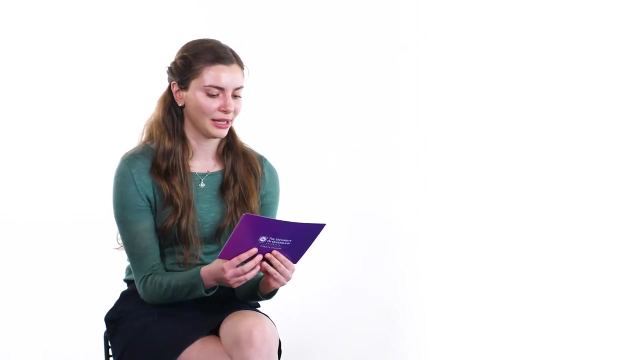 Hi, I'm Ron. I'm a lecturer in environmental and marine science here at UQ, and I'm here with Laura, who's a student in environmental science, and we're here together to answer some of your questions. Looks like I have the first question. So what is it about UQ's approach that makes us the most employable graduates in the state? 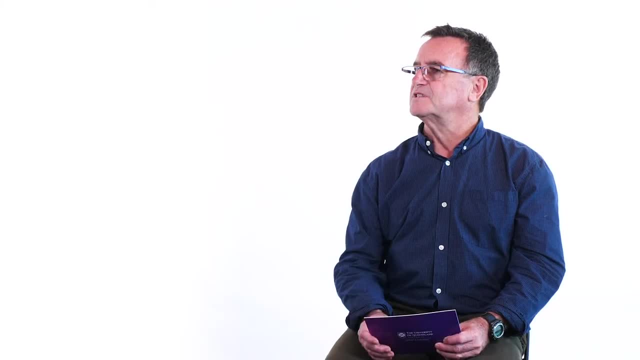 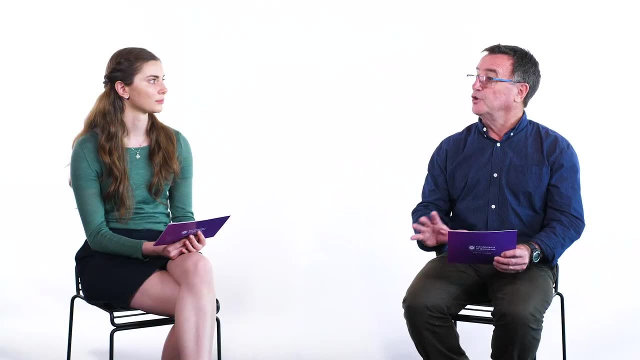 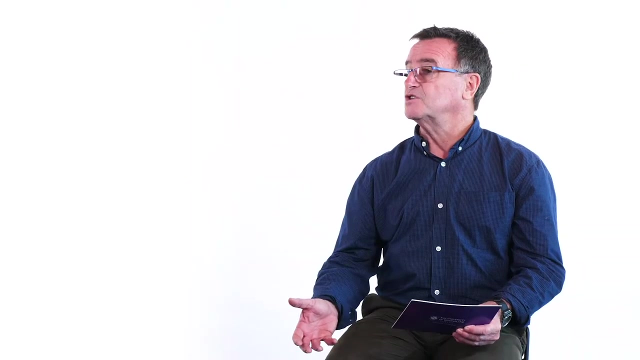 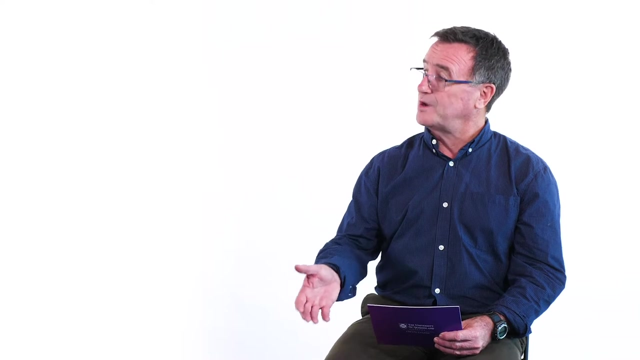 I think, in the centre of it all, it's the integration. It's the integration of the technical, the academic knowledge and all of that learning, but it's integrated heavily with exposure to industry, with exposure to people who will actually potentially employ you. And so we have a number of courses, for example, where you on the one hand, do an internship, where you literally go and work in an office, work in industry, with the people who will potentially be employing you. 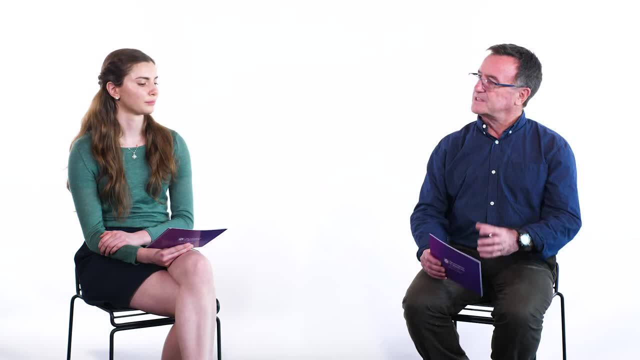 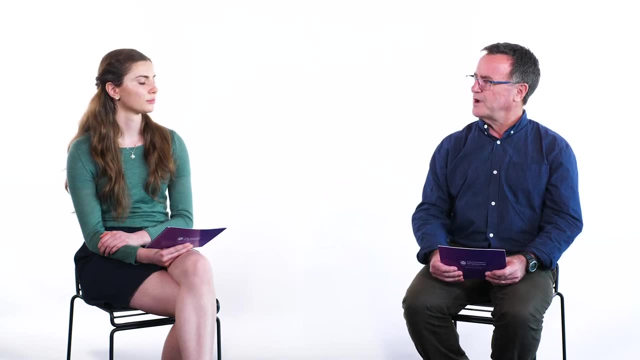 And so you really learn the sort of on the job skills and at the same time all of the technical academic work is tailored to dovetail into that, and so there is a very strong effort to integrate those two, if you like, sides of what you learn at UQ. 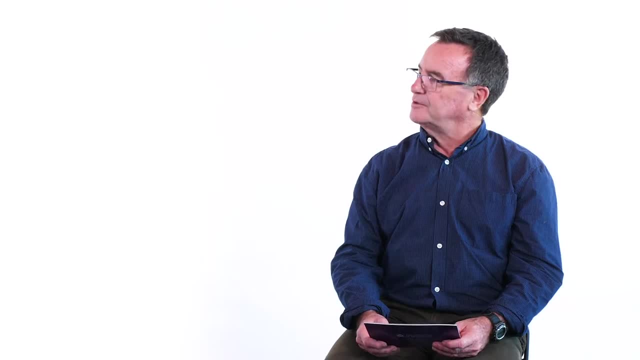 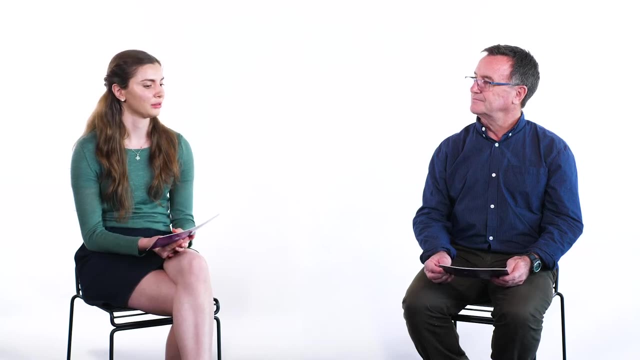 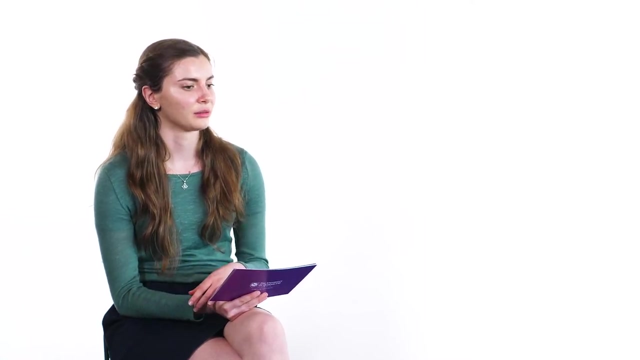 What does a day in the life of an environmental science student look like? A day in my life would probably start with some lectures in the morning, maybe based on biology usually, And then we have three hour practicals from there where we look at plant biology or soil science, and then some more integrated tutorials in the afternoon, and then some more lectures to top it off. 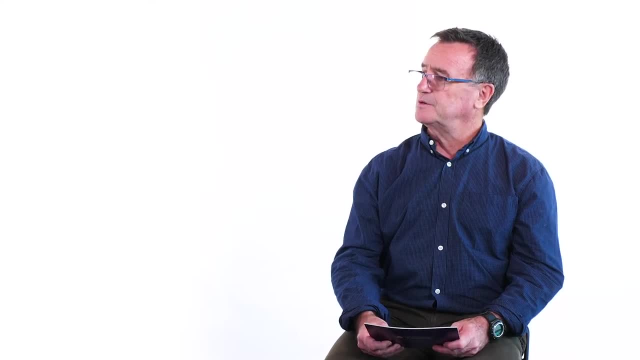 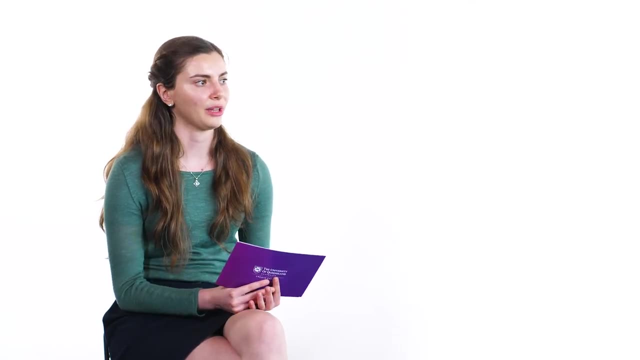 What is the most interesting thing you've learnt? that has not been part of your coursework. The most interesting thing I would have learnt would be from one of the seminars I attended through UQ. So we had something that was talking about the underwater volcanism and the processes around hydrothermal vents. 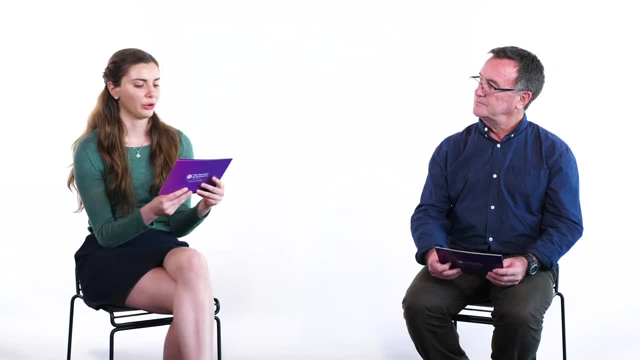 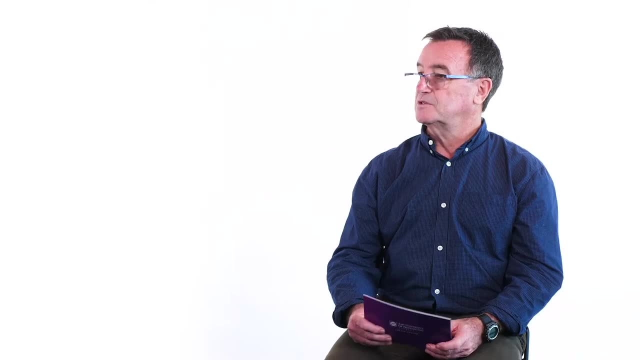 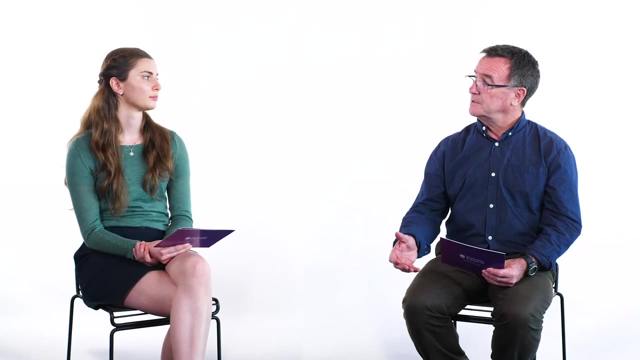 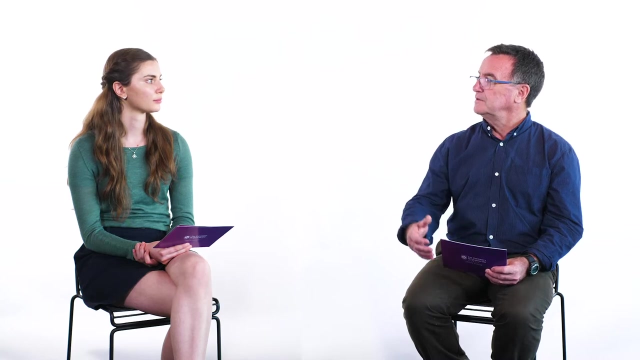 So that was really interesting as well. What opportunities do your students have to get hands on experience in our industry? There are a number of courses where students are proactively exposed to industry and that can be where they undertake a team effort to solve a real problem for a real partner, a real client. that might be a local government agency, or it might be a not for profit management or environmental group. 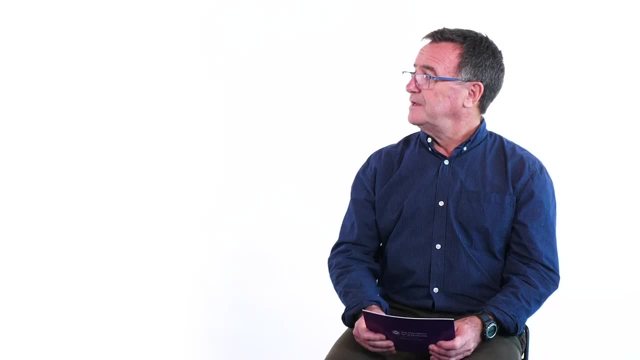 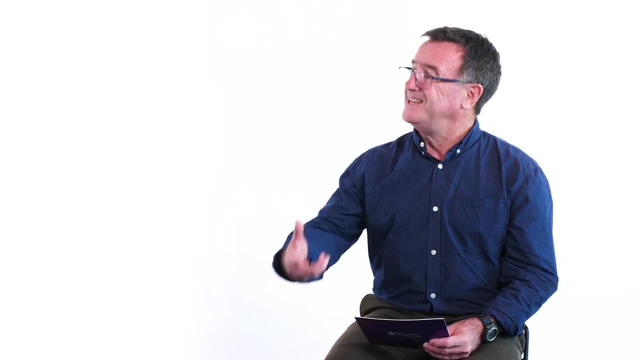 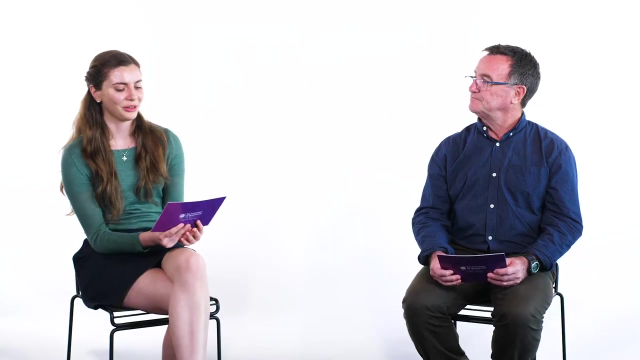 But at the same time they then also have the chance to participate in an internship where they are actually placed in industry and they work at the tasks in the job that they might aspire to do. What are some of the coolest jobs your former students are doing? 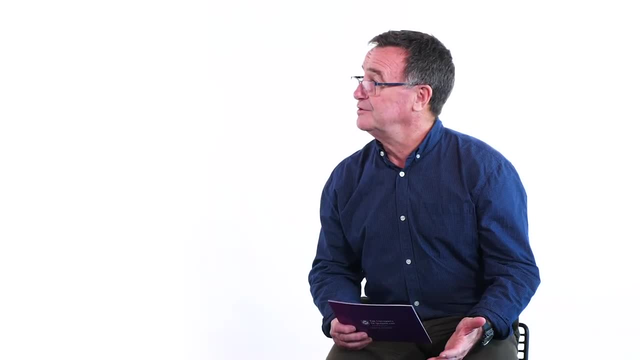 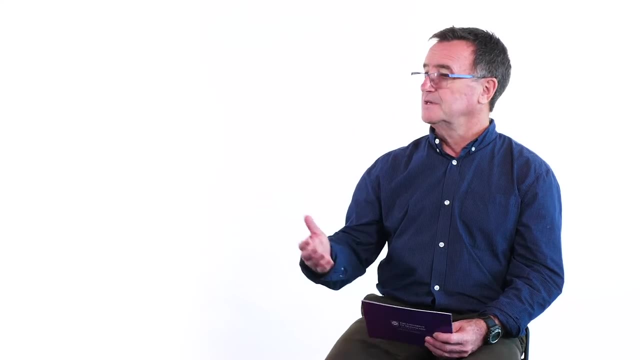 Well, I have a number of students that have gone off to do some really interesting things, So some of them, of course, have gone off to work in consulting companies For local government, for state and federal government. For example, one of the students is now working for the Auditor Generals in Canberra. 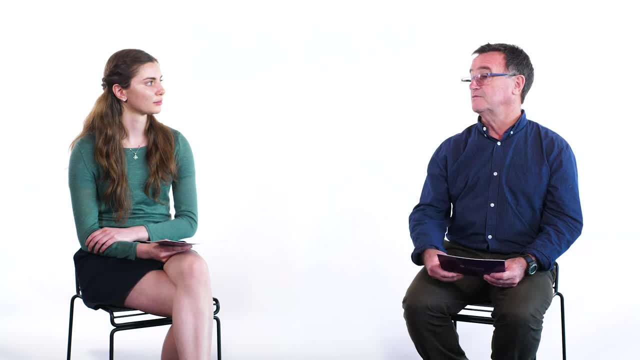 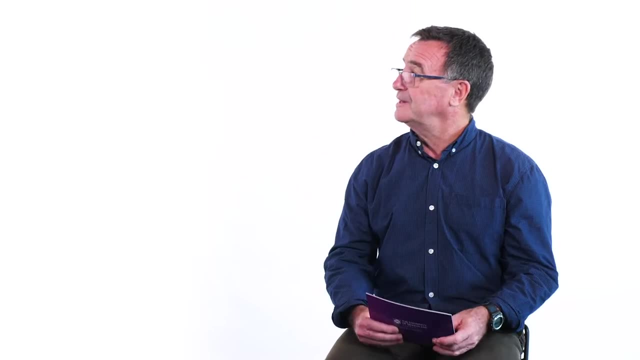 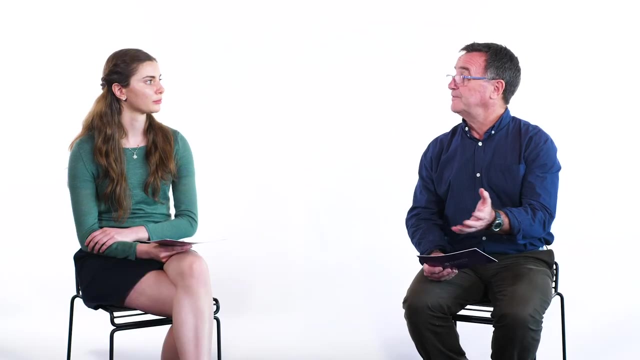 At the same time, some of the students have gone off. there is one that has gone off and worked for WWF. There is another one who has gone off to work for the Pew Foundation, which is an international philanthropic foundation supporting environmental issues, And then, of course, there is another student that went off and is currently working for the United Nations Environment Programme. 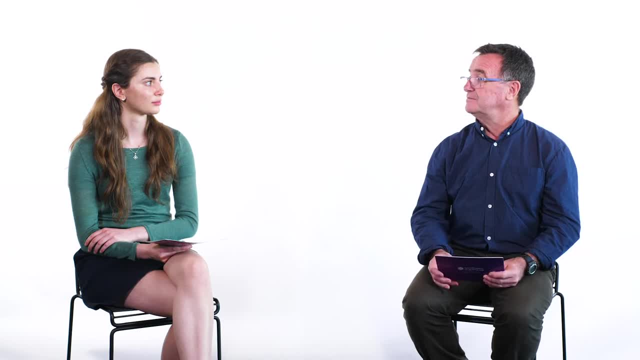 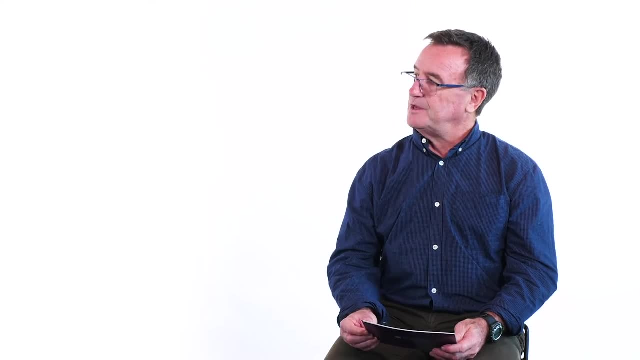 So there is a whole range of opportunity out there that students seem to be quite easily slotted into. Yeah, it sounds quite amazing. What are the most valuable skills you have learnt as part of your degree? Some of the most valuable skills I would have learnt would definitely be some of the hands on practical experience we get. 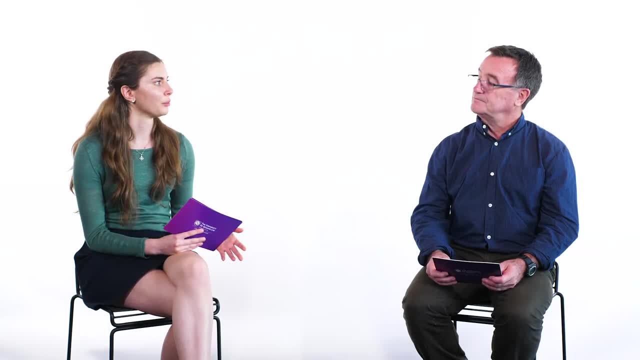 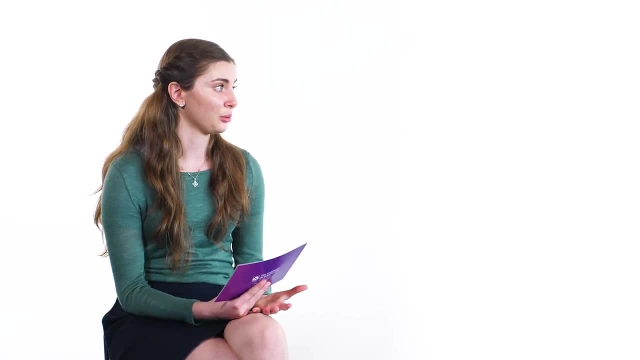 So I never expected the amount of field work that we do get to do with UQ, as well as the laboratory techniques that we get to learn. So it is really valuable the statistical knowledge I now have, As well as some of the problem solving that we have done in classes with hands on work. 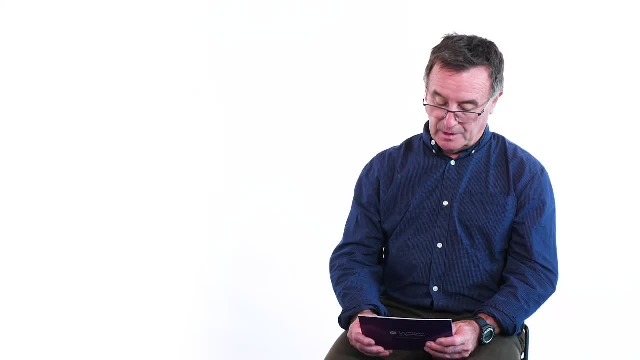 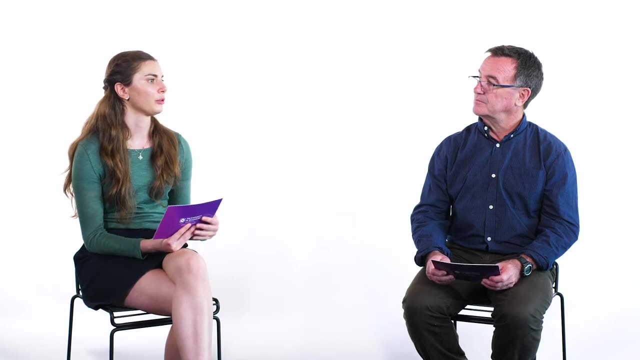 What do you think employers in your industry are looking for? How do you think UQ has equipped you with these skills? Some of the most important skills I think employers would be looking for is definitely work experience is one, So we have different internship opportunities through UQ, as well as some work placements that we can find in the programs. 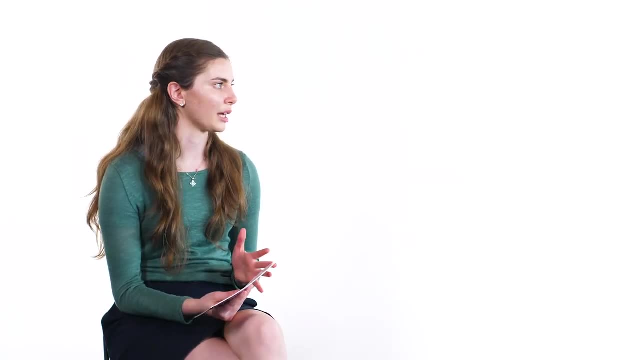 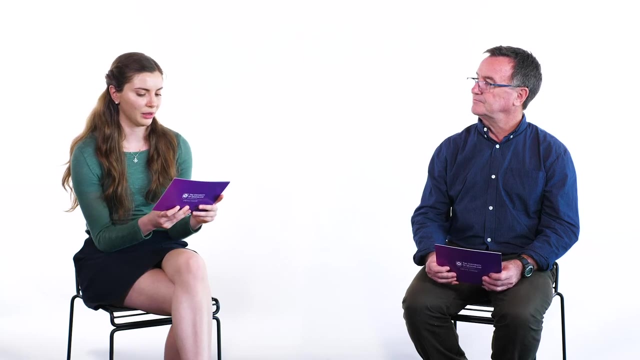 And other things would definitely be the communication skills that you get through UQ Group projects, as well as some of the solo work you can do with research as well. If you could give me one piece of advice that would set me apart as a job candidate, what would it be? 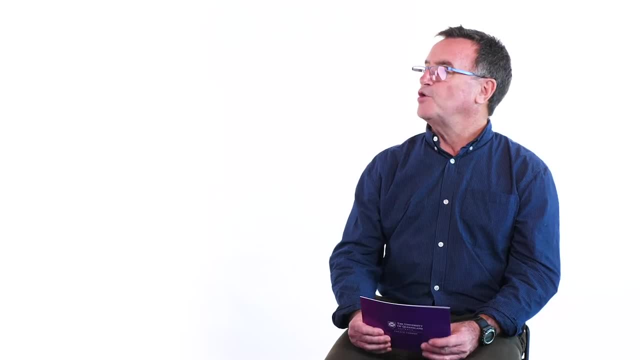 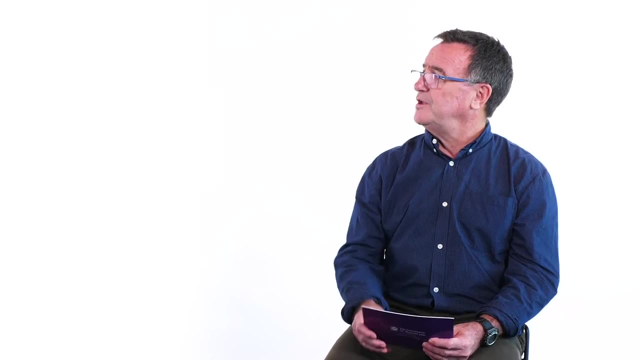 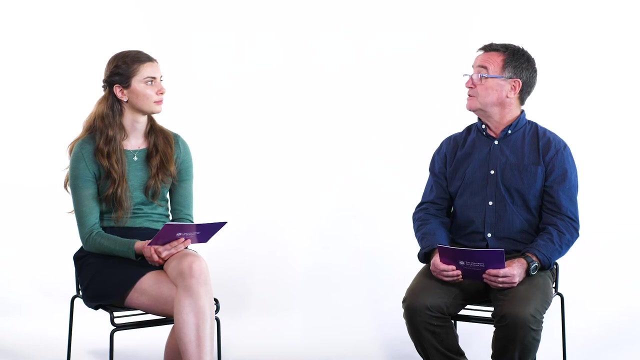 I think it is to be open minded in your approach. Of course, in any interview you have to be clear and you have to be up front with what you know and really make obvious what your strengths are. But in general terms I think you have to be open minded to solving problems in new and different ways.